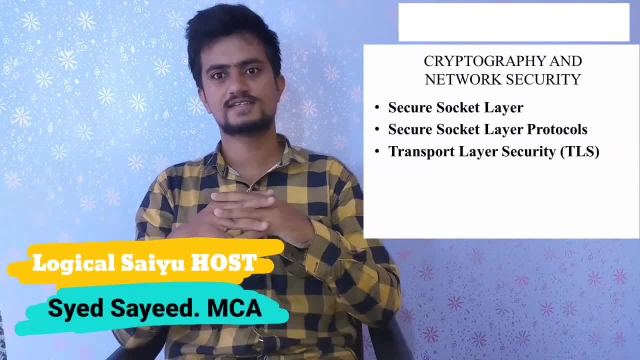 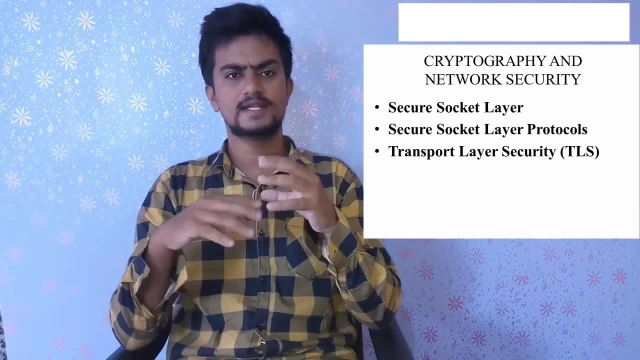 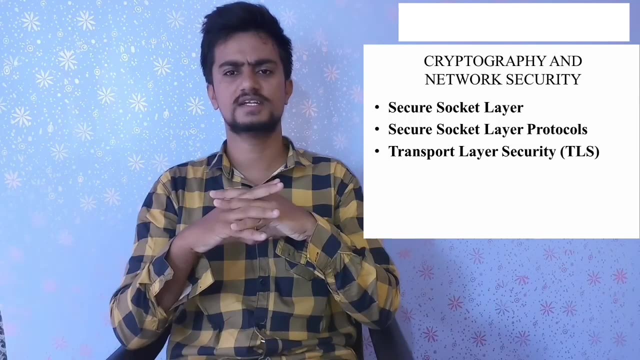 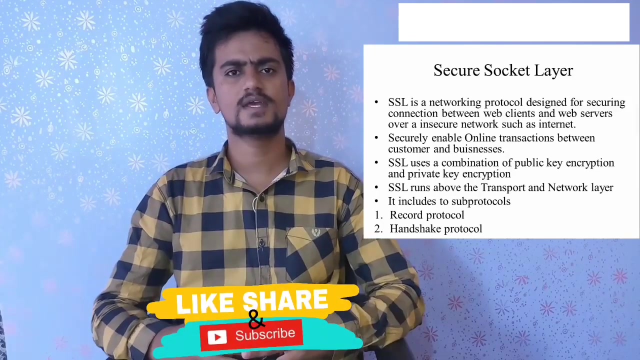 So hi, hello everyone. Welcome back for logical sayo Friends. today we are going to discuss a one of a type of topic that is nothing but secure socket layer and different types of protocols in secure socket layer and transport layer security. So these three topics we are going to discuss in detail today. So let's start. So what do you mean by secure socket layer? Secure socket layer is nothing but a. it is type of protocol and designed for a purpose of secure socket layer. 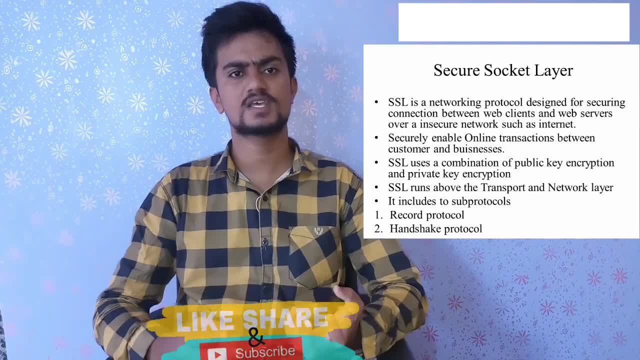 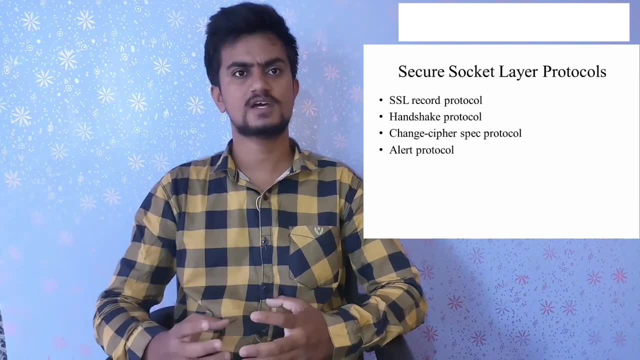 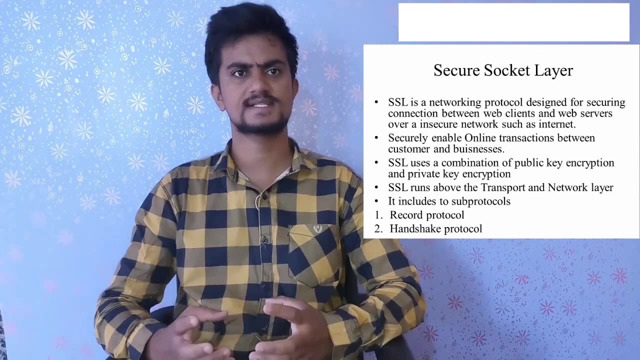 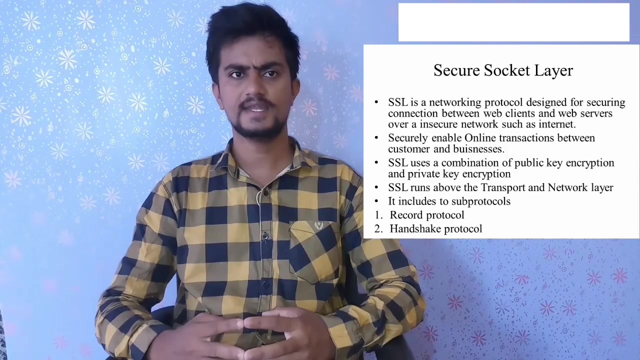 Secure communication between web client and a web server over an insecure channel such as internet understood and it enables online transaction. It enables online transaction from customer to business. The best example for this is Amazon flip cop. They are using this SSL certificate and they have given trust, built a trust on customers by using this SSL certificate and next coming for SSL users, a combination of both private key encryption. 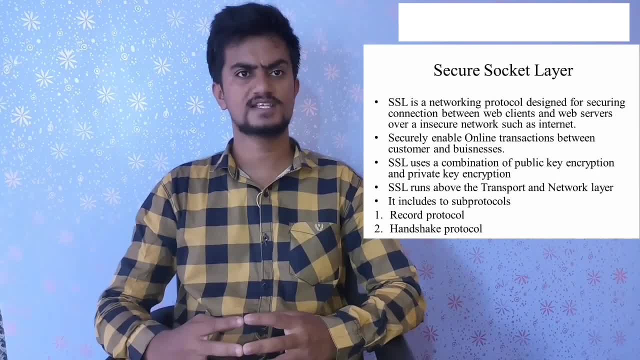 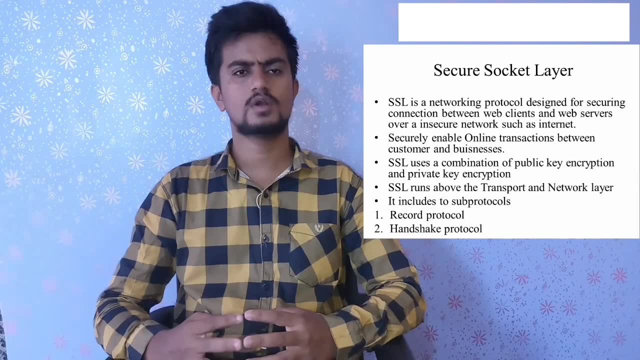 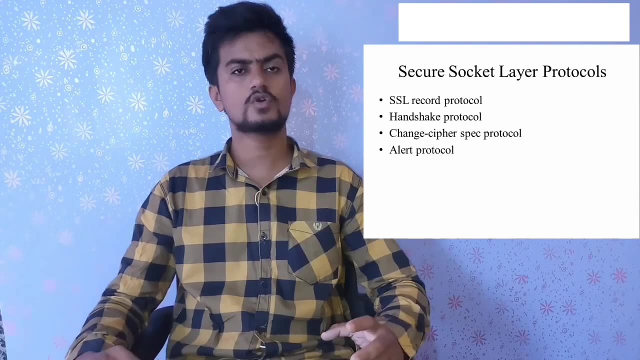 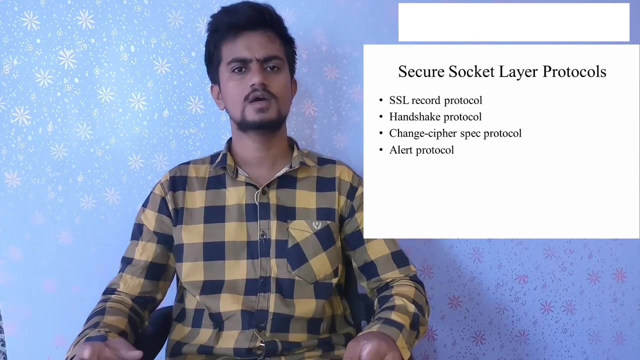 and public key encryption. This SSL runs above the transport layer and network layer and it has two sub protocols that are handshake protocol and record protocol. understood and next is different types of protocols in protocols. in SSL means secure socket layer. There are four main types of protocols that are SSL: record protocol, handshake protocol, change cipher. 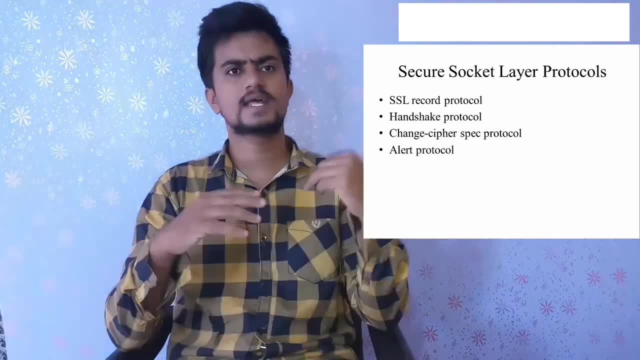 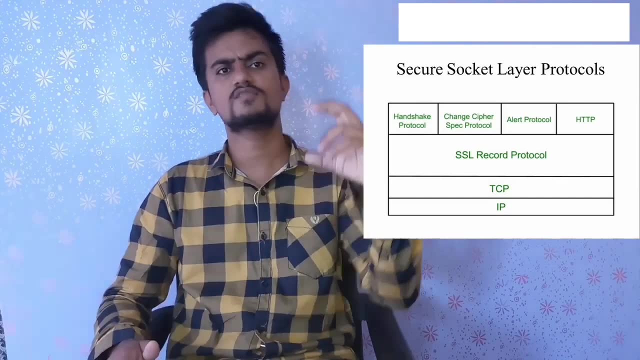 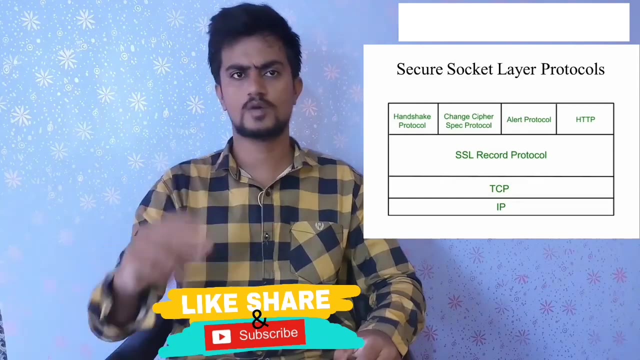 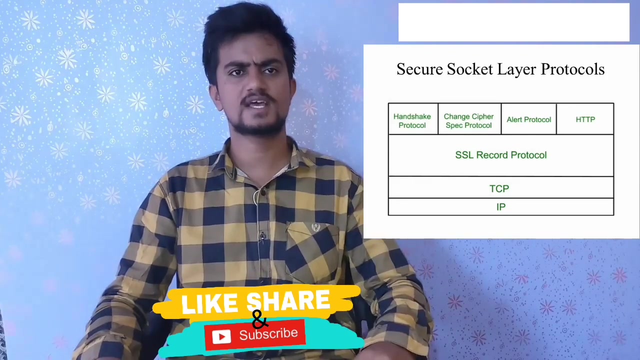 spec protocol and alert protocol. So, as you can see, the diagrammatical picture of this SSL protocol, this in this cryptography. we are going to read the diagram not from a top to bottom, but bottom to top. we are going to read this diagram from a bottom to top. understood, the first layer in this is IP internet protocol and next layer is TCP transmission control protocol and, above that, SSL record protocol and the top. 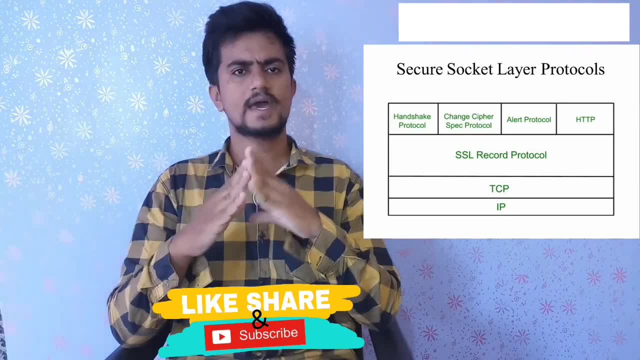 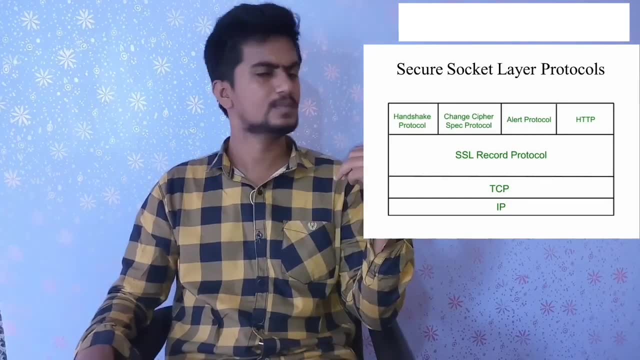 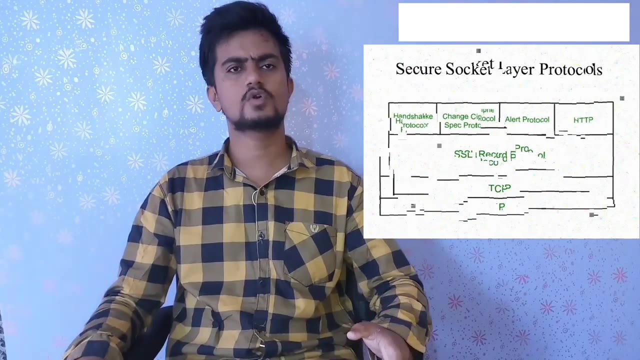 layer is divided into four sub parts, that is, handshake, protocol, change cipher, spec protocol, alert protocol and HTTP. This diagram is understood and next, coming to detailed discussion of this SSL record protocol. This protocol has main two services to this provides two services of SSL protocol understood. the two different types are confidentality and integrity. 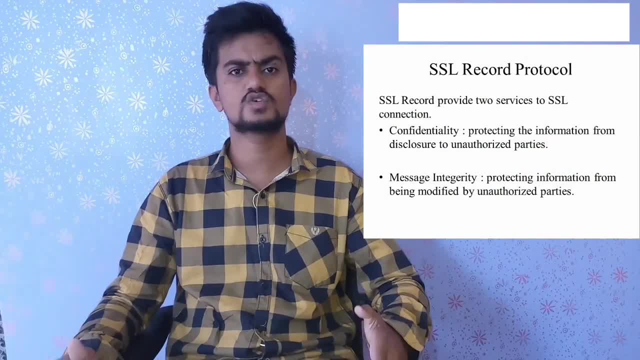 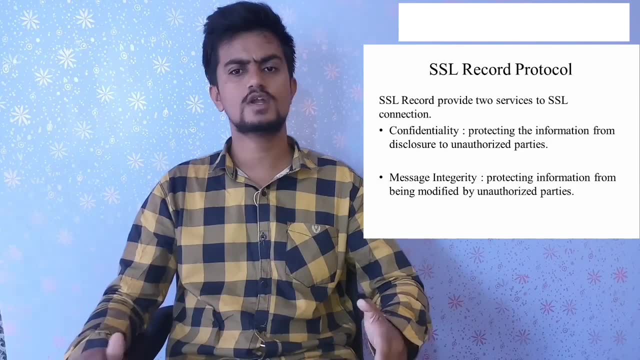 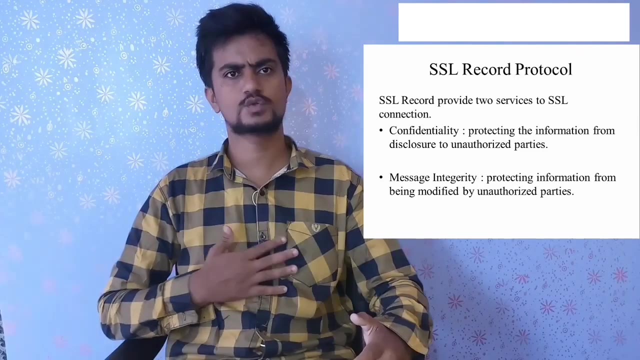 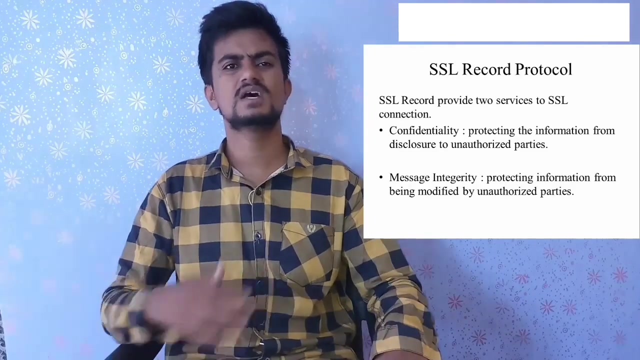 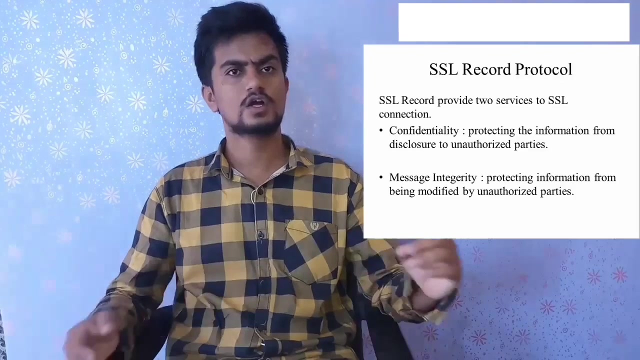 Confidentiality means protecting the information from the disclosure of unauthorized parties understood, and integrity means protecting information from modifying the unauthorized parties. means confidentiality means our personal data should not be publicly published by someone. That is nothing but confidentiality. Integrity means our own personal information should be modified or edit. correction should be done by ourself, not should by any third parties understood. These are the two major services provided by SSL protocol. 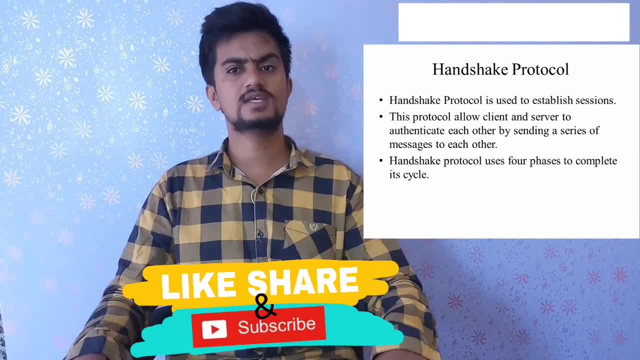 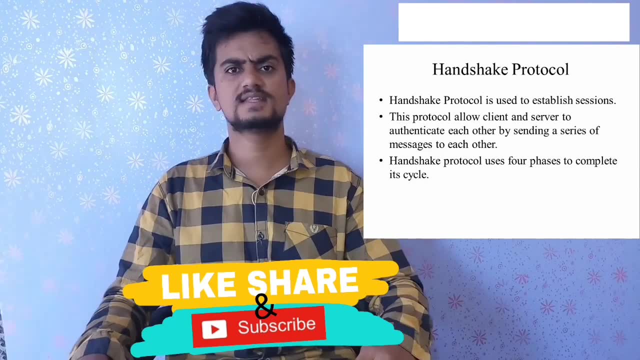 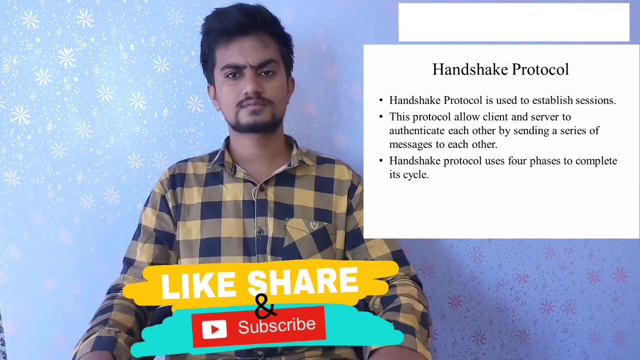 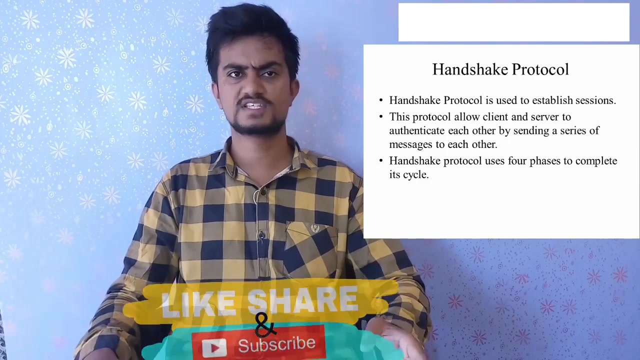 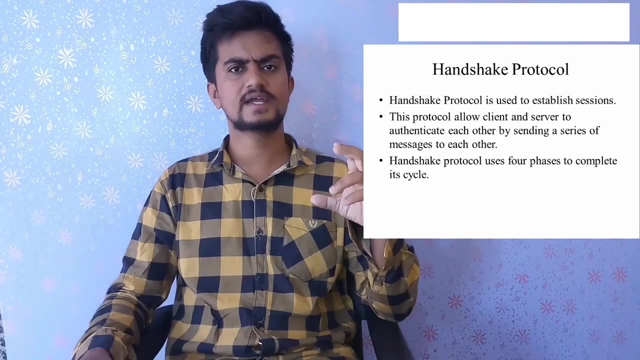 And next is handshake protocol. Handshake protocol is used to establishing a session. Session is a one of a main important topic. Session is nothing but when client and server communicates with the client. That is nothing but session. This protocol allows client and server to communicate between each other by using message passing understood. Take example of Facebook login system. If we give our credentials correct- username, password- then only it will allow us to access our FB account. 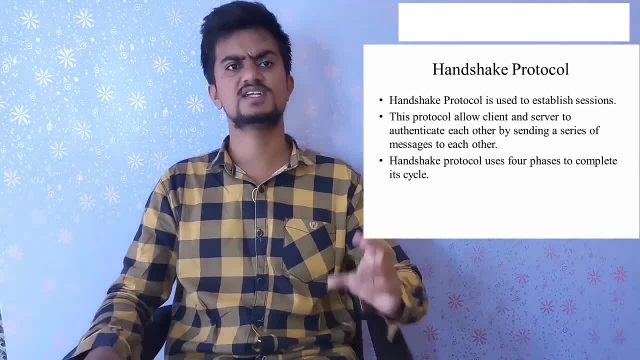 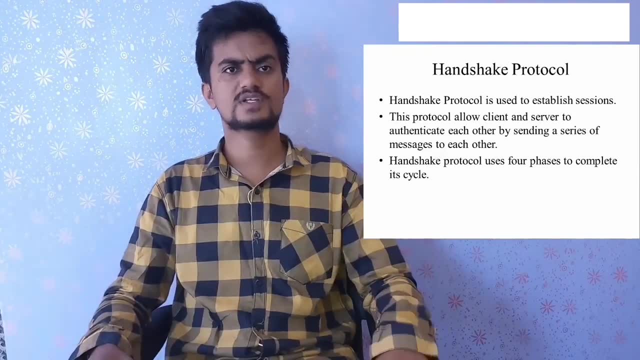 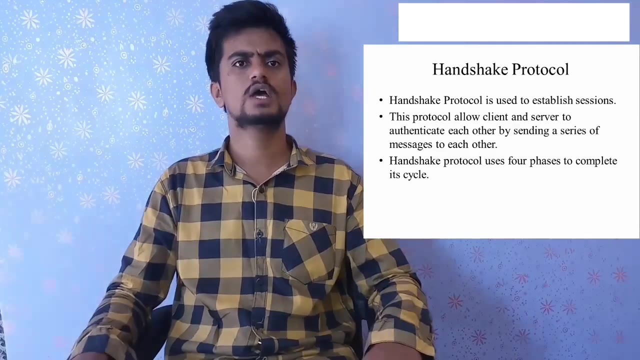 If we have not given correct password means it will display error message. That is nothing. but it has session when client means I, You also client when you interact with your own personal FB. that is server. understood. Handshake protocol has main four different phases. that is, phase one, phase two, phase three and phase four. understood. 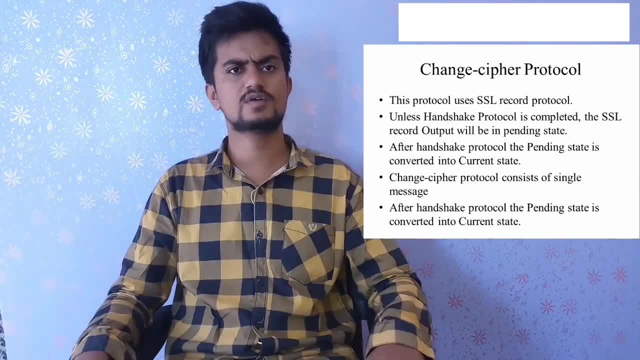 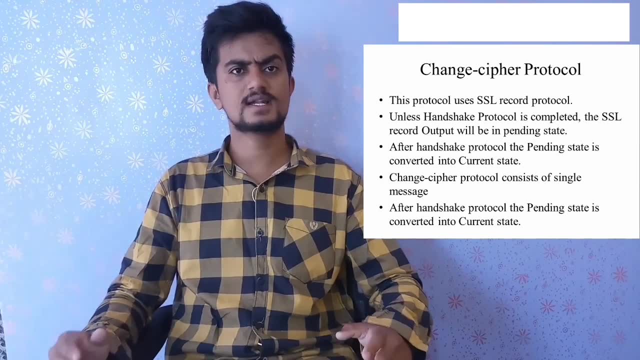 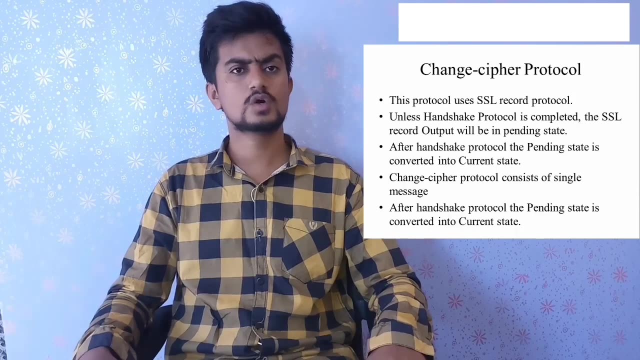 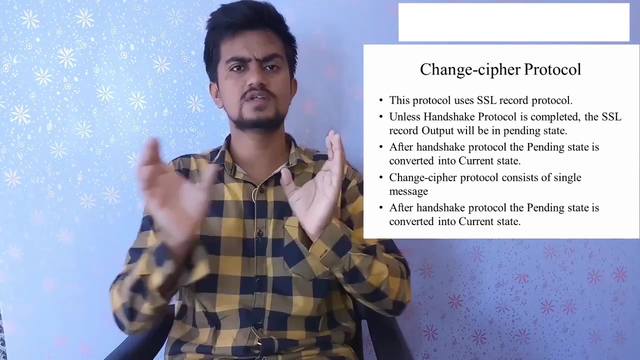 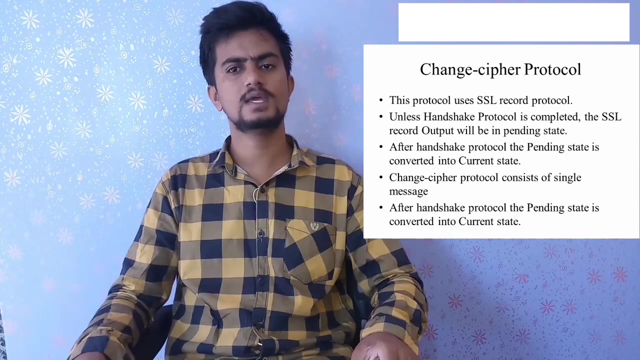 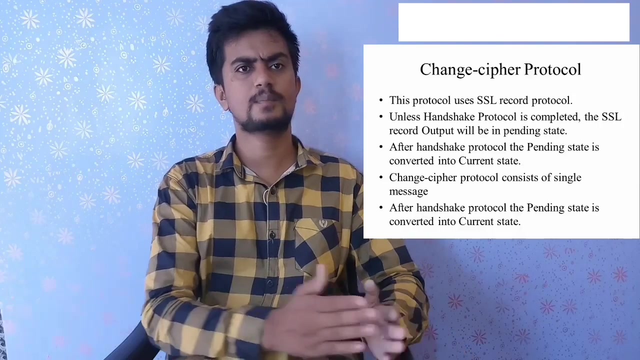 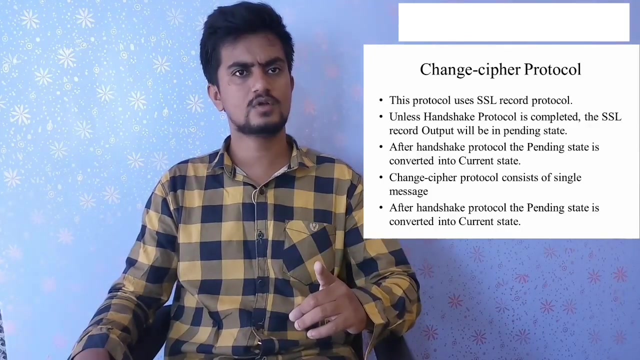 And next coming for change cipher spec. This is a also a one of a type of protocols in SSL. that is, this protocol is used to SSL record protocol. understood This protocol is used to SSL record protocol. So from that time you are, You are also observing a one word protocol protocol. So what do you mean by protocol? protocol is nothing but agreement between two different parties, understood. Unless a handshake protocol is completed, the SSL record output will be in pending state after handshake protocol. Once you use handshake protocol, it will change the pending state or it will change the output from a pending state to current state. understood Why we use handshake protocol. 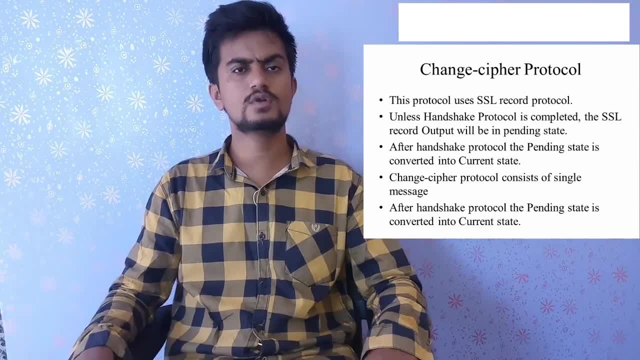 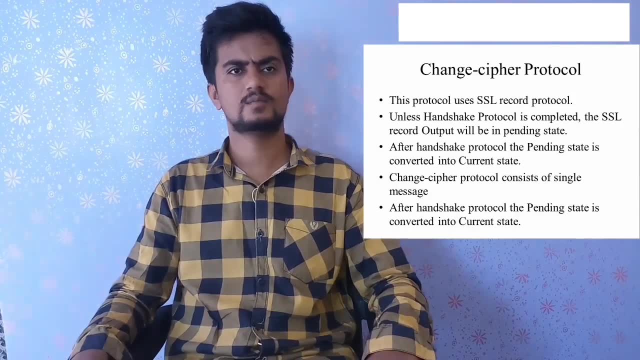 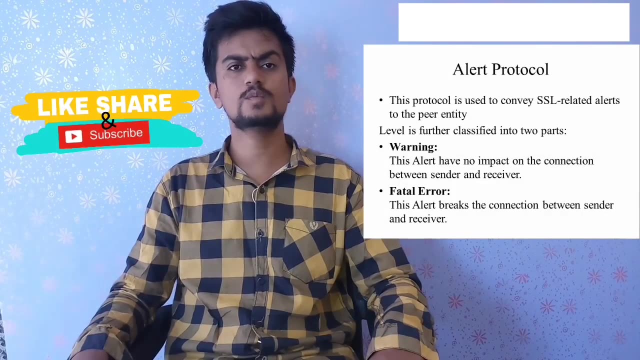 Handshake protocol used for a changing the pain output from a pending state to a current state, understood, and this chain cipher spec has one single message, that is one byte. and next coming to last protocol in this is alert protocol. what do you mean by alert protocol? what do you generally be alert something? 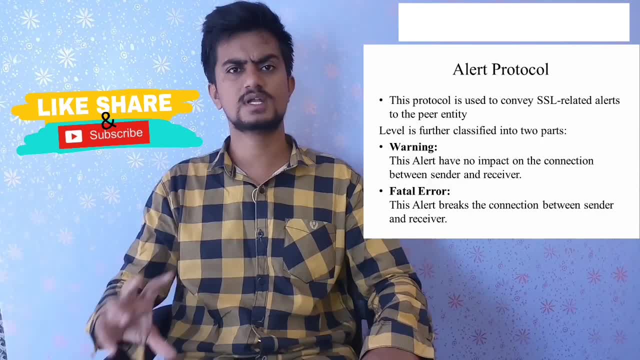 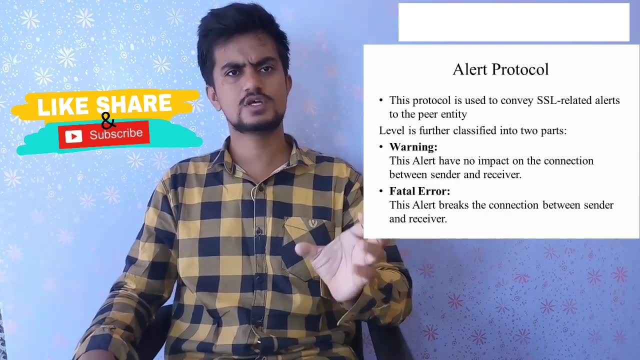 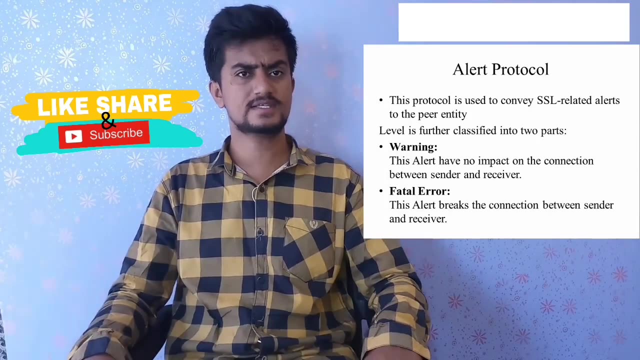 going to be happen that is dangerous to us is nothing but alert generally. next, coming to this, official definition of alert protocol means this is also one of a type of protocol. it used to convey the ssl related alerts to peer entities. it is used to convert the ssl related alerts to. 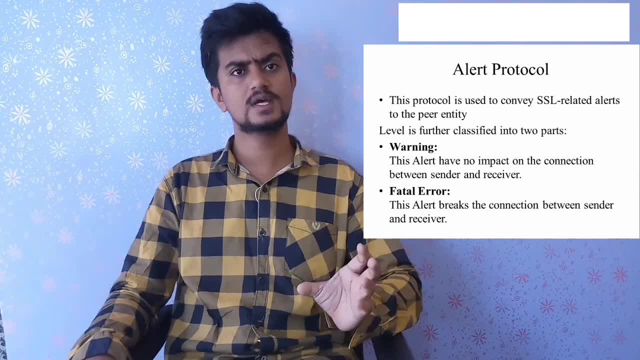 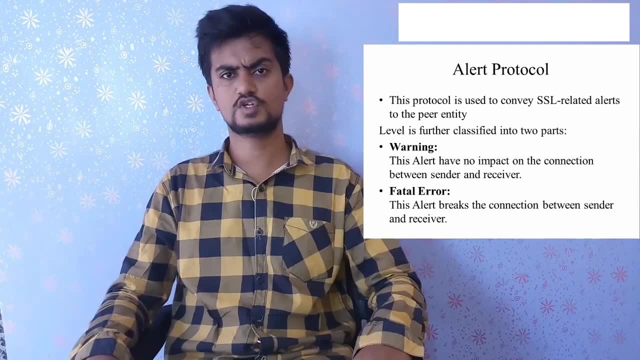 your peer entities. what do you mean by peer entities? what do you mean by fear? peer is generally nothing but person to person communication, understood. fear is nothing but person to person communication. in this system, no client will be there and no server will be there in this there. 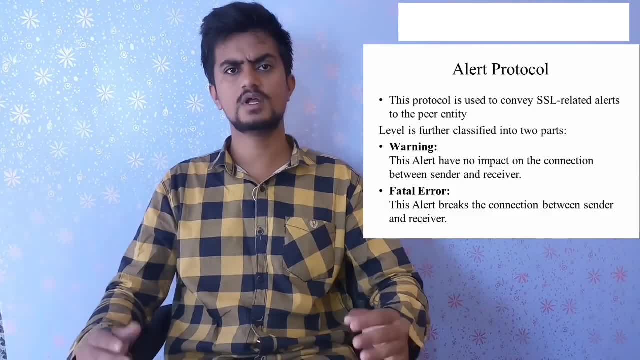 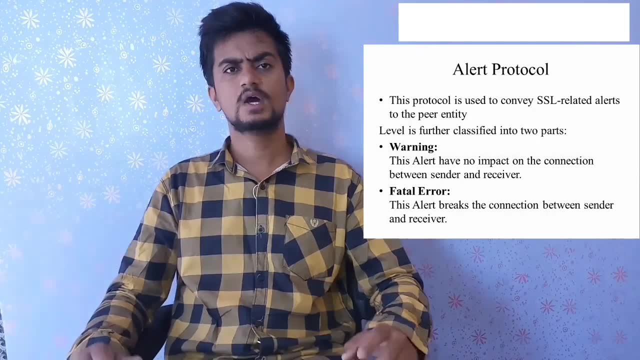 are levels are further classified into two types. in alert protocol it has been further classified into two levels. that is nothing but warning and fatal alert. so what do you mean by warning? warning is nothing, but when you and client and server are interacting with each other, it doesn't break its. 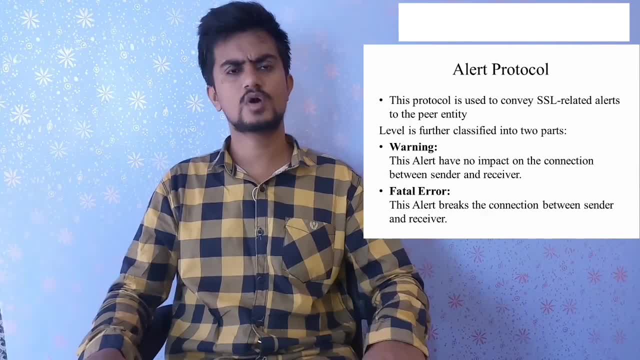 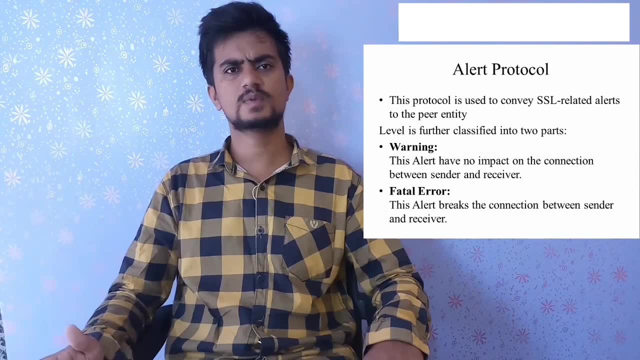 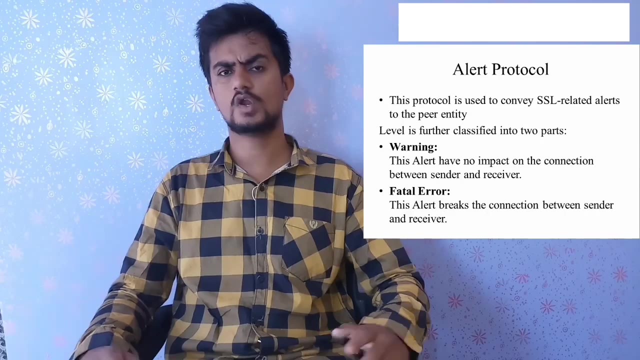 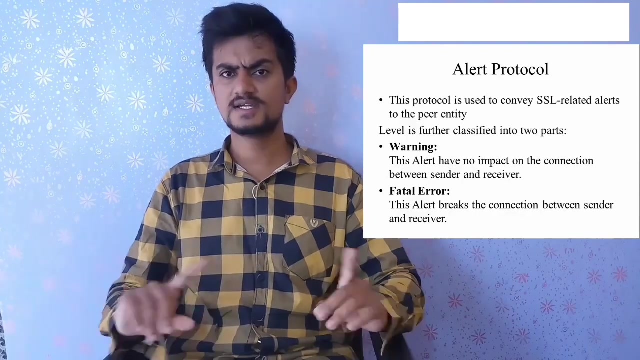 connection. it is nothing but warning. take example for a warning: while you are using your whatsapp or anything, certain message will become from your friend, so it doesn't don't take that example. take another example, example of facebook. when you are using a facebook or youtube- best example, youtube- while you are watching a youtube, suddenly will got a message in whatsapp. 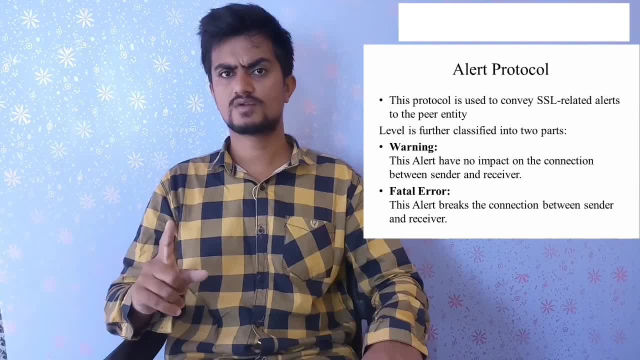 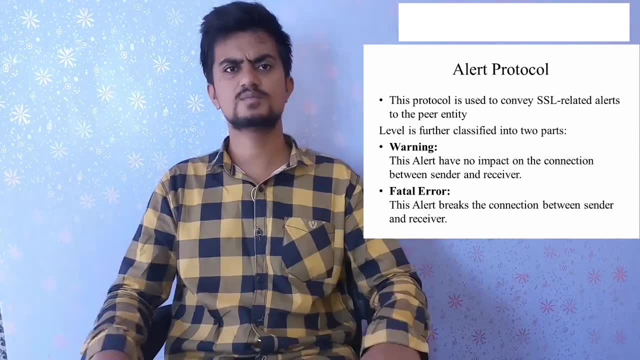 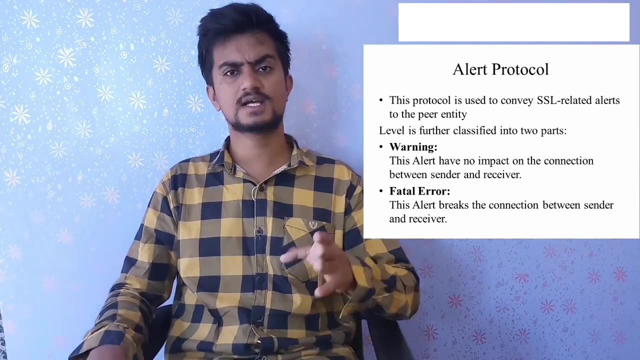 it doesn't breaks its connection. are you observed? your youtube video will be not cut or it doesn't come to home. the video will be running. the message will become: it doesn't break you and youtube client and server. that is nothing but warning and fatal error. what do you mean a fatal error? it breaks. 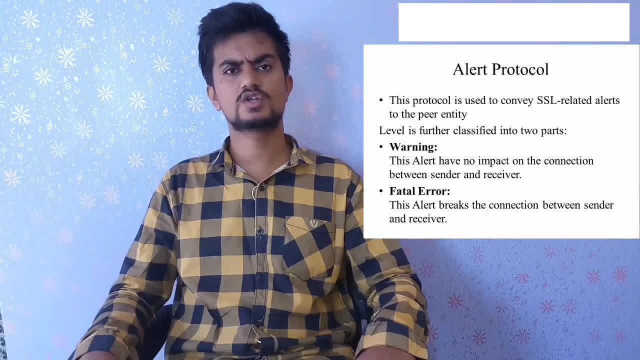 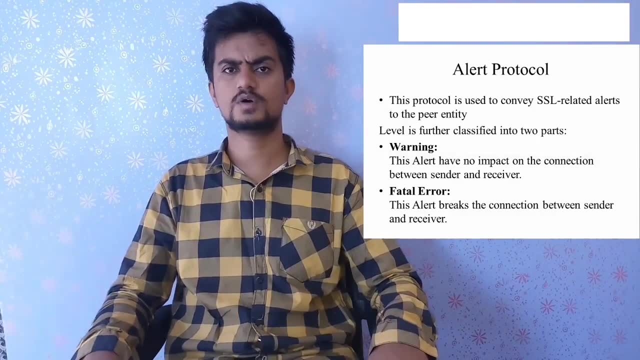 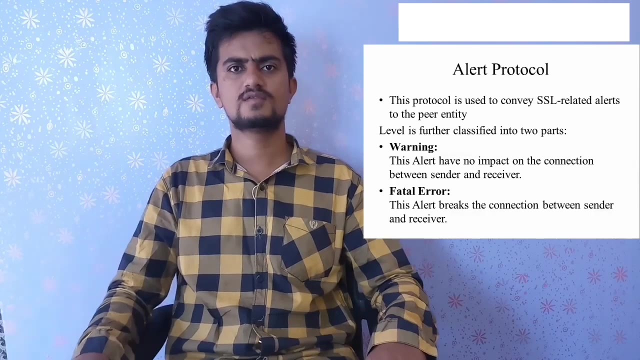 between client and server. take example, while you are using youtube or facebook, only when you drag your phone above to below, then you have put your mobile phone in flight mode. then your connection will break. no, that is best example for warning. so these are the about two levels that we have discussed. and next, 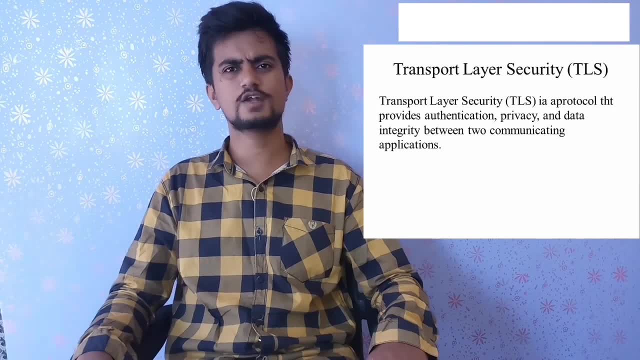 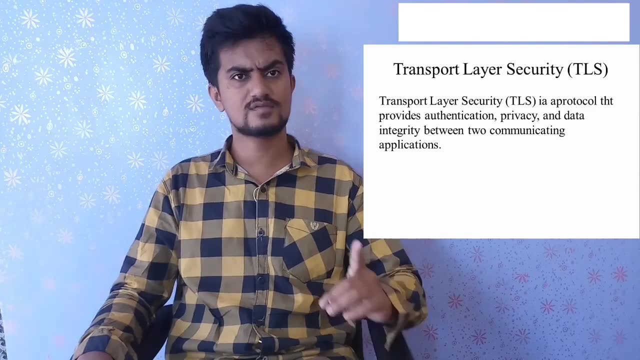 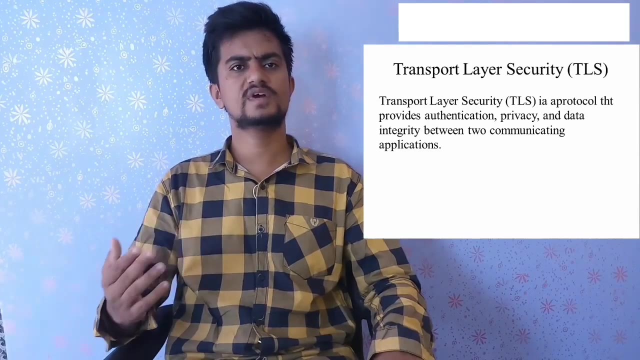 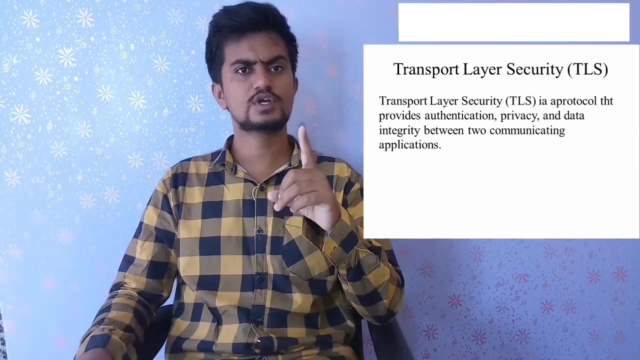 coming forward. one of the main important topic is transport layer security. transport layer security: it stands for TLS. it is a one of the most important protocol in cryptography and network security. it a protocol that provides authentication, privacy and integrity between two communicating parties. understood, transport layer security provides a security. provides a security. 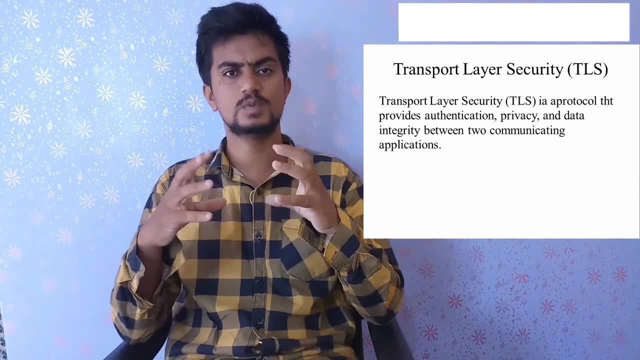 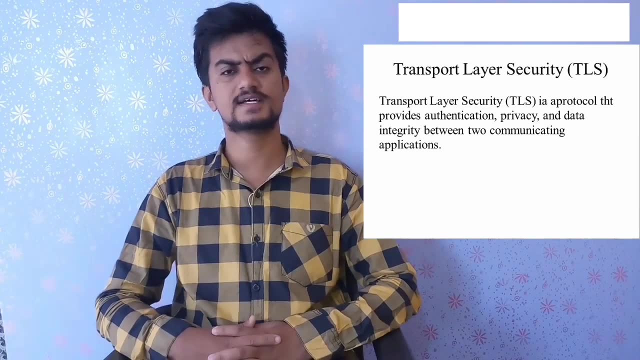 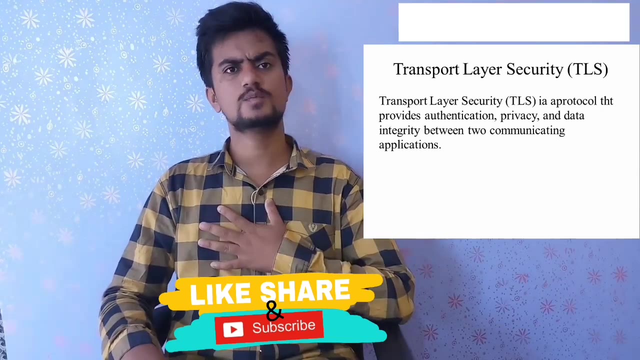 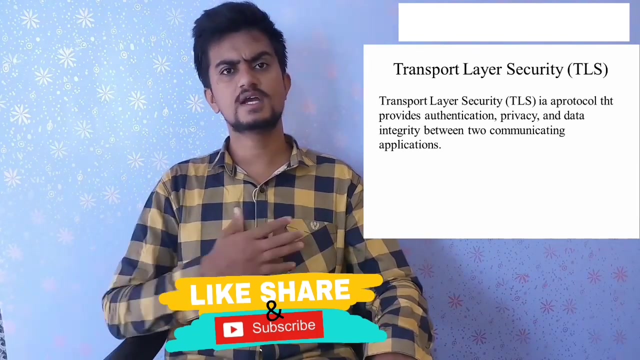 of privacy, authentication and integrity between two communicating parties and communication education. take a real, real-time application example for this transport layer security as facebook. while you are using Facebook, let comfort privacy. privacy means what do you mean by privacy? they take as a way or your Facebook account only well, editing our personal. 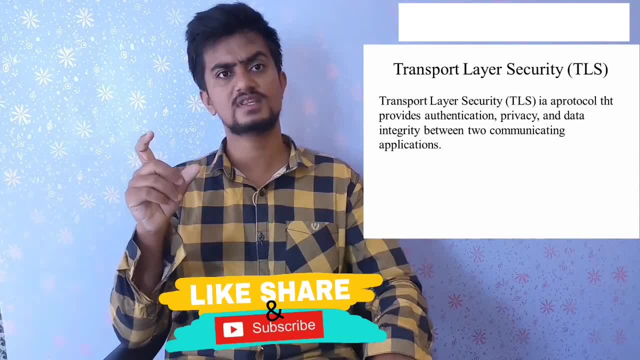 information. I kept my year or date of birth in that other. I kept to my Year of Born as Year of Born, as only me. that is not only an example of transport layer security. we did another one as you learn: all objectives for transport layer security. only if there is oneworking you can use this. we keep the ihr date of work in the data, but I kept my year of born as year of born, as only me, that is. 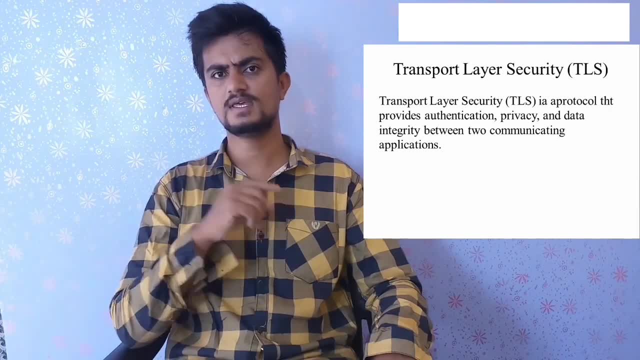 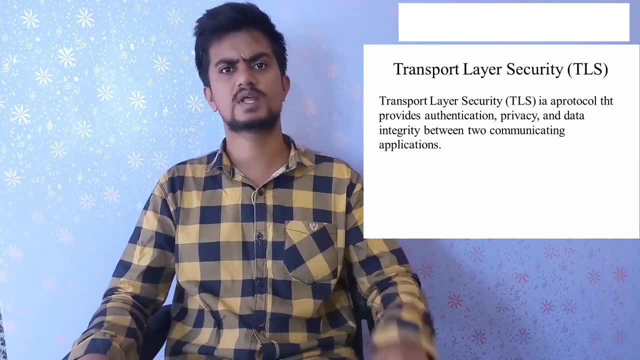 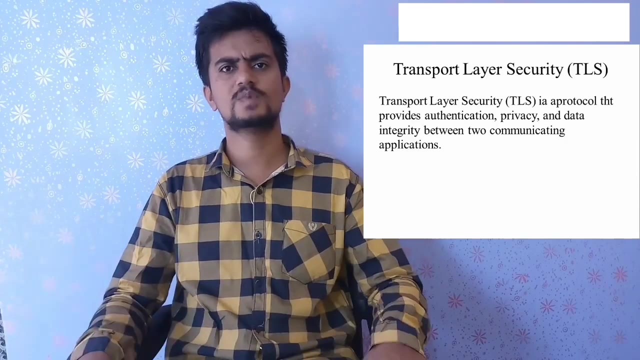 nothing but best example for privacy. in this my year of birth is seen or view only by me. no, it is not disclosure publicly. that is nothing but privacy. and next, coming for authentication. authentication means the correct user should log into his account. means once we provide our correct username and 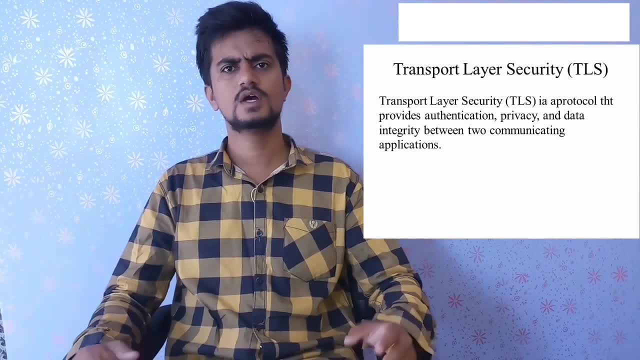 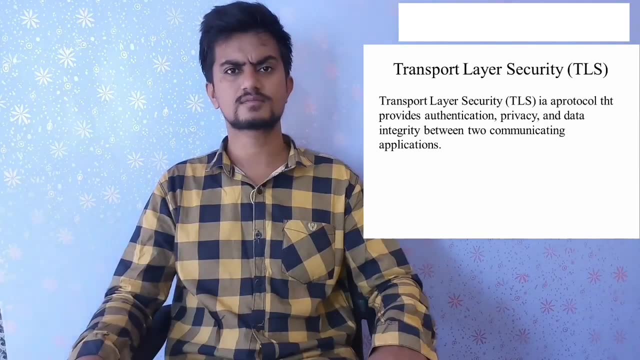 password. then only we can log into Facebook account, our instead of. if you have given a wrong username or password, it will not allow us to login. that is nothing. a best feature: by using this transport layer security, the unauthorized, unauthorized access- third parties could not access to our account. next, coming to 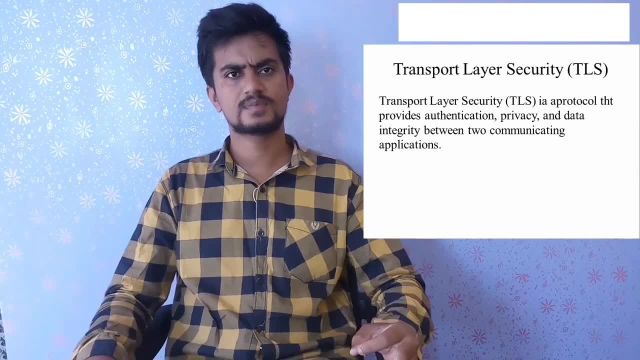 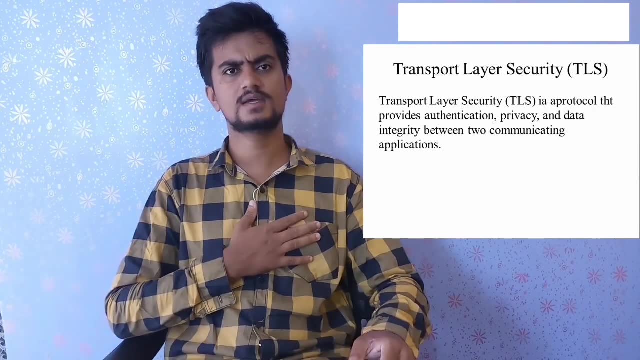 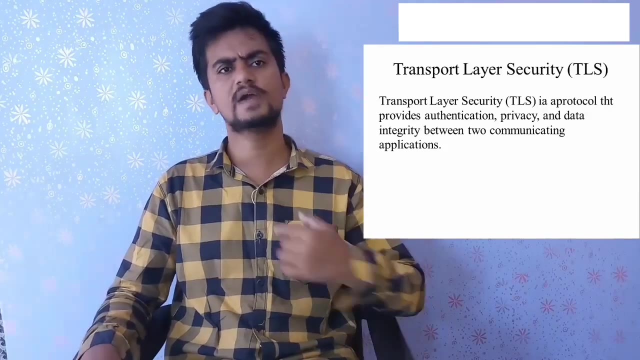 integrity. integrity means the data should not be accessed by any third party. understood the my facebook ID or my facebook post should be posed by myself only, not by any third parties, not by any third parties by you. your account should not be edited or posted by my. my account should not be. 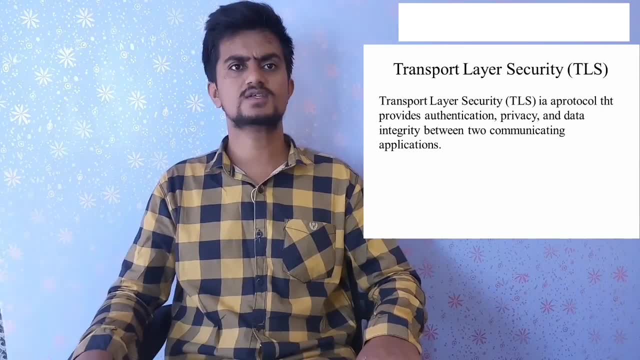 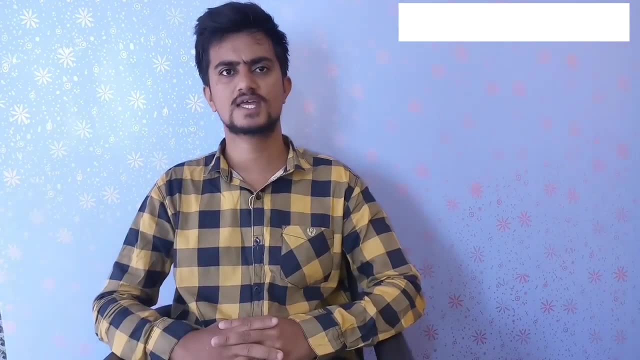 posted by yourself. that is understood. that is nothing but integrity. so I hope you have been understood. if I have been understood clearly, then subscribe my channel. I hope you have been understood, so thank.